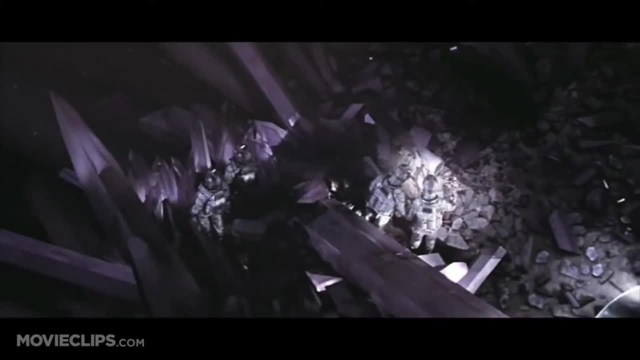 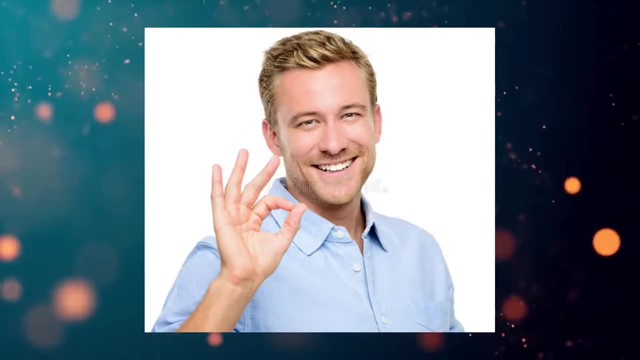 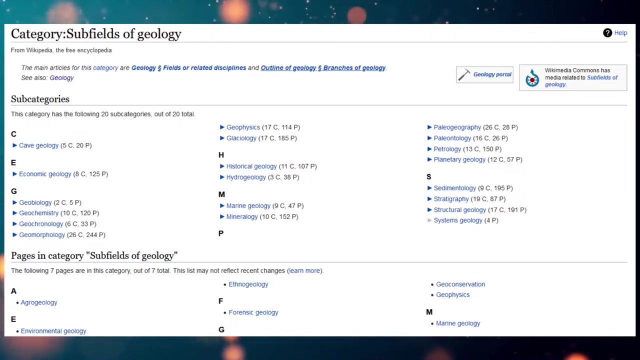 perhaps earthquakes? Well, yes, that might be some of it, but there are other fields just as important as well. I am going to flash you an image of the subfields associated with geology. Ready, Here it is. As you can see, it is quite a lot. You got economic geology, geochemistry. 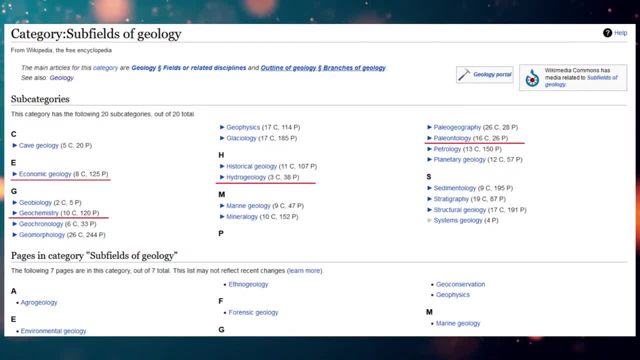 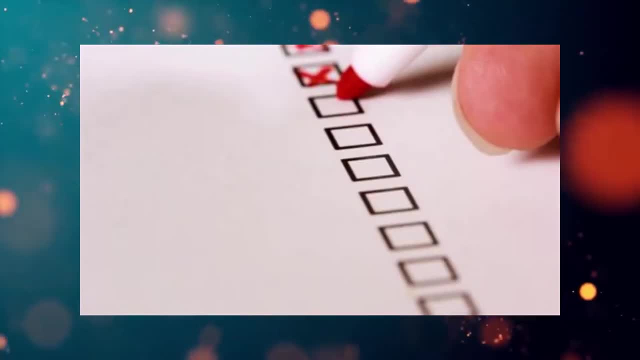 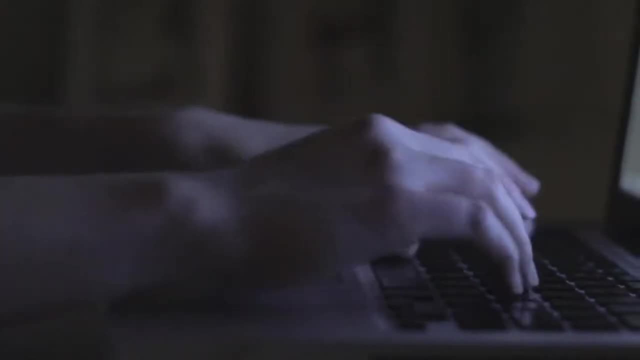 hydrogeology, paleontology, sedimentology, volcanology and so much more. The list might not even be complete. With the emergence of new technologies, the field of geology gets more diverse and new specializations start to appear. We will talk about some of the few notable fields mentioned earlier. 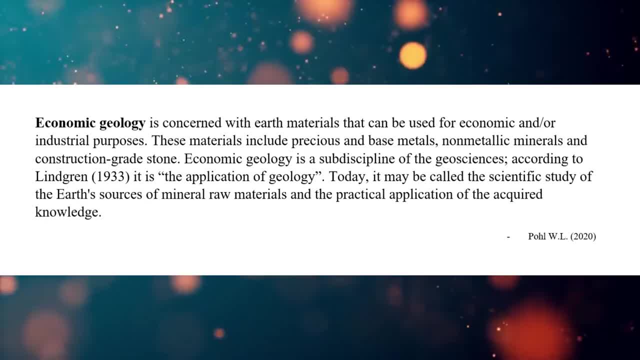 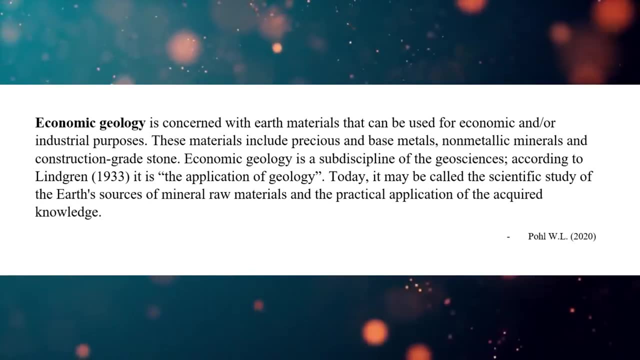 First is economic geology. Economic geology is concerned with the earth's materials that can be used for economic and or industrial purposes. These materials include precious and base metals, non-metallic minerals and construction-grade stones. Economic geologists are the ones 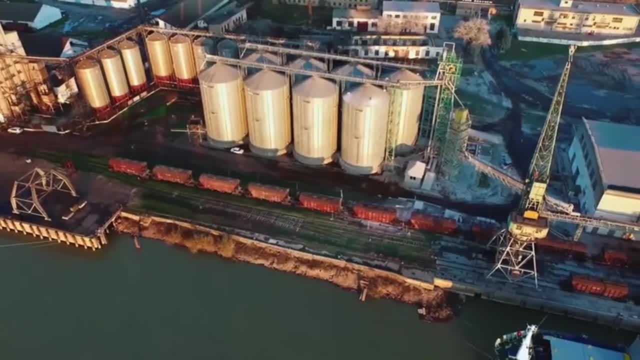 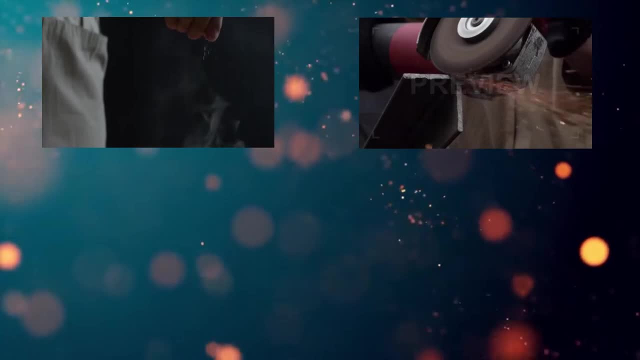 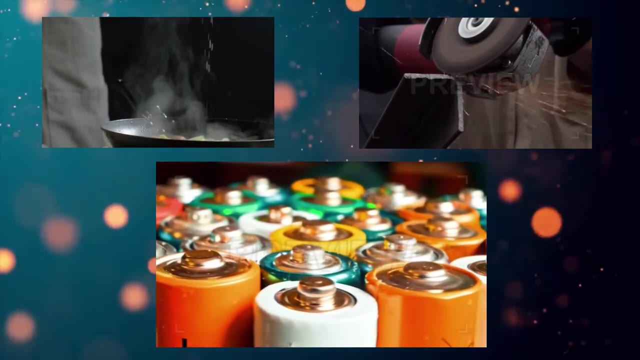 responsible to find areas which have economic value and have resources that can be mined for use. The salt you put in your food, the metal used in construction manufacturing and the batteries are all thanks to economic geology. Next on our list is paleontology. 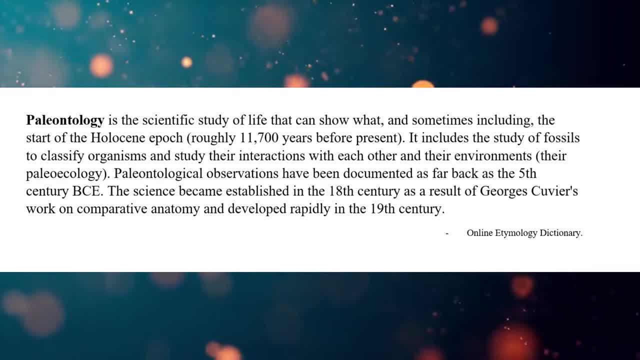 Paleontology is the scientific study of life that can show what, and sometimes including the start of the Holocene Epoch, roughly 11,700 years before the present. It includes the study of fossils to classify organisms and study their interactions with each other and their environment. 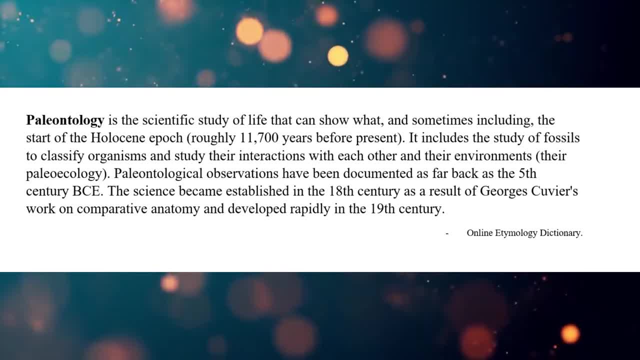 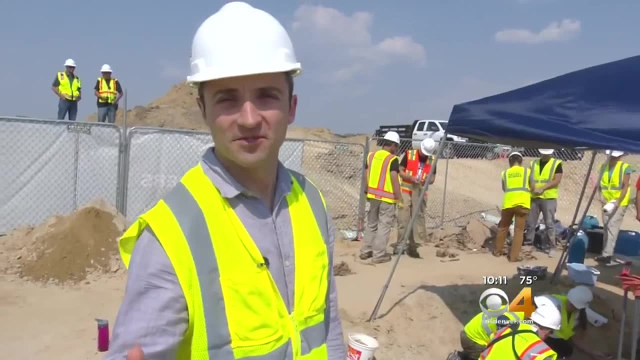 or their paleoecology. Paleontological observations have been documented as far back as 15th century BCE. Paleontologists are the ones responsible in digging up rocks, using them to relatively date rocks and perhaps speculate what is life millions of millions of years in the past. 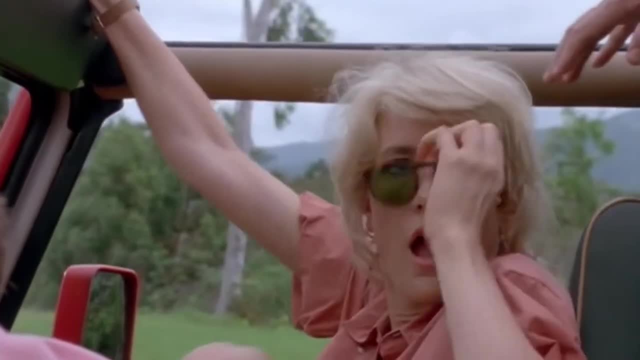 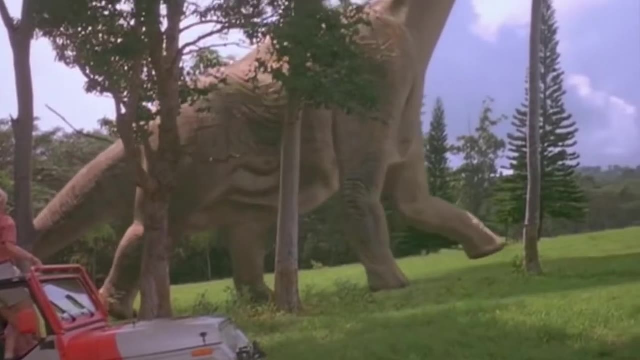 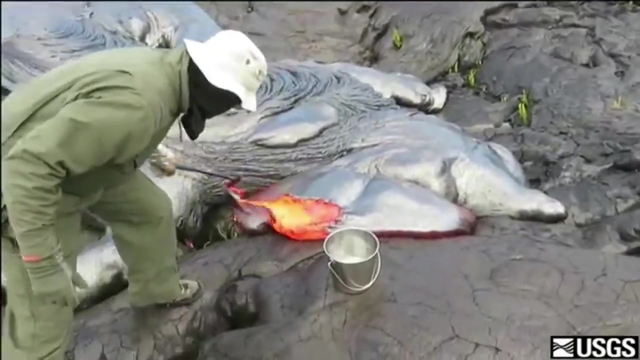 The reason why we have dinosaurs in pop culture references is thanks to this field of geology, Volcanology. And lastly, we got volcanology. Yes, that's right, one of the most popular and well known fields of geology. But what is volcanology?